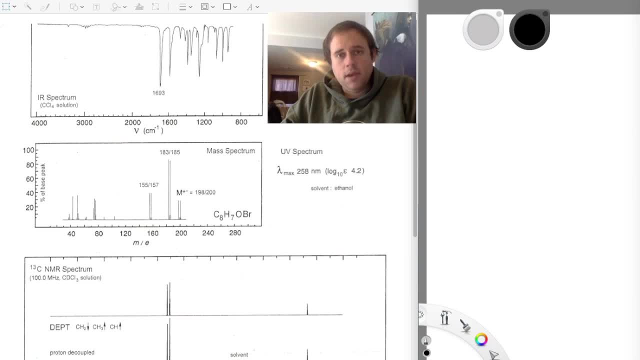 will utilize IR, so we use infrared spectroscopy, mass spec. sometimes we can utilize UV-Vis, although we tend not to do that quite as often. and then we certainly have NMR, And NMR is the large one that is sort of held above the others, because it is vital in determining. 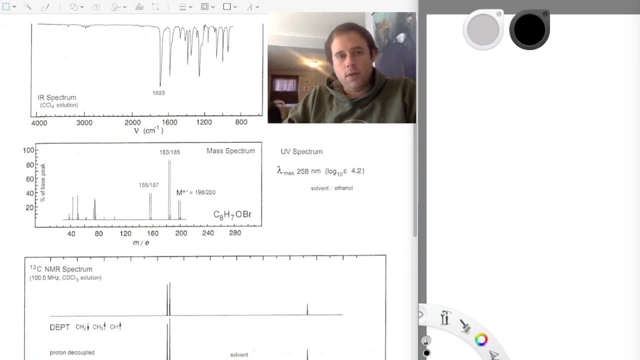 the skeletal structure of the organic compound that we're working with. So what I thought I would do- and this will probably be a series- I don't know how many of them I'll actually get uploaded today, but I will continue along with this to give people practice What I'd 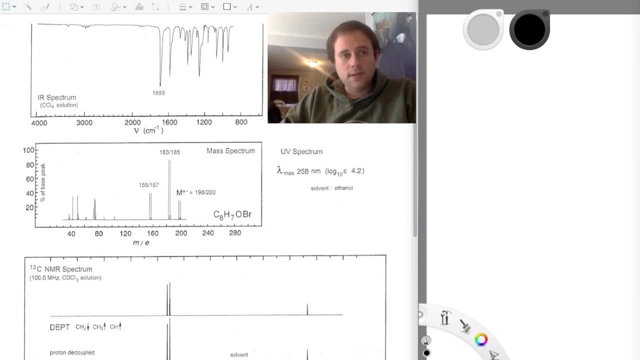 like to do is: I would like to present potential unknowns- and they will be accompanied with an IR, a mass spec and a carbon and proton NMR- and then attempt to solve for the unknown, Because this is really a lot of students are faced with this challenge in organic chemistry. 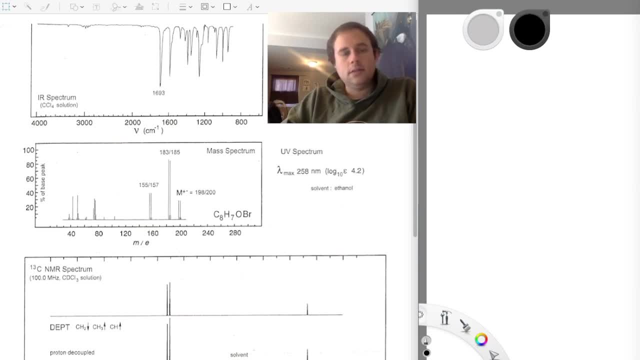 too, and they tend to struggle when they're trying to solve these. So I'd like to take a look at this and sort of walk you guys through what pieces of information are vital and how I would go about solving one of these and approaching this And, like I said, we'll 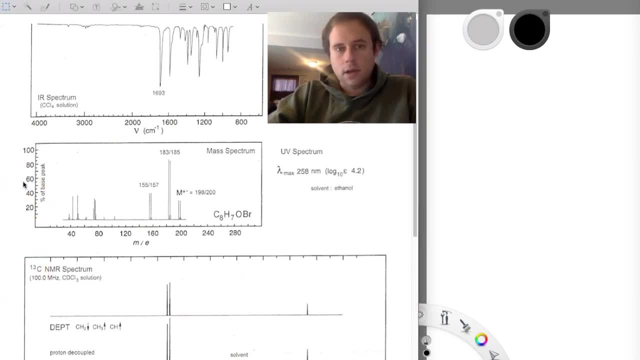 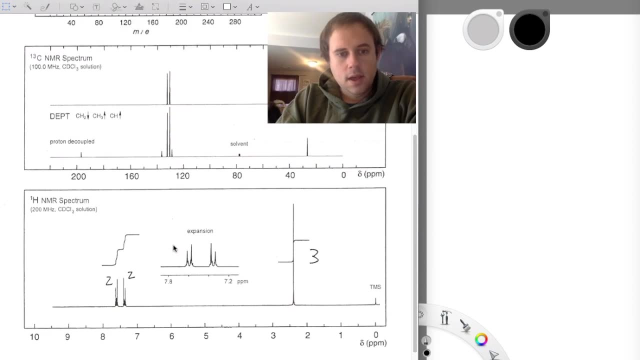 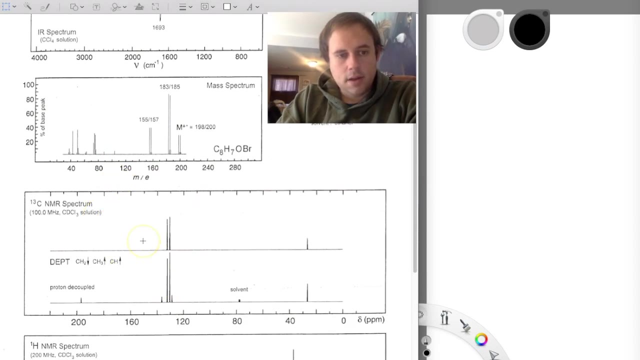 try to do a couple of them, Alright. so if you take a look over on the left hand side, here we have the various spectra that we will be dealing with. So I'm going to go back up, but the order here is: we have IR, then we have mass spec, we have our carbon 13, NMR. 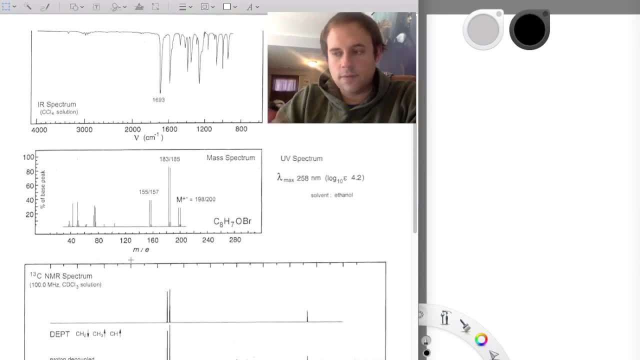 then we have the proton NMR, And I will talk about each one of these in turn, Just as a sort of disclaimer notice. this is not going to be teaching the ins and outs of NMR spectroscopy or IR mass spec for that matter. So if you are looking for videos on that, I do have. 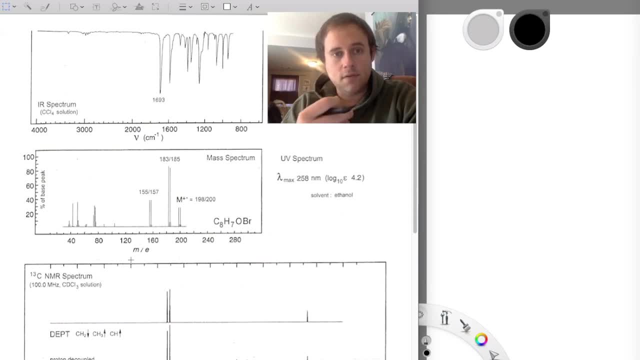 videos that explain chemical shift and deshielding and integration. I don't know if I have a video on splitting. I should probably make one of those soon- But you should be informed about how to read NMRs. This is primarily going to be how to solve them, But the general 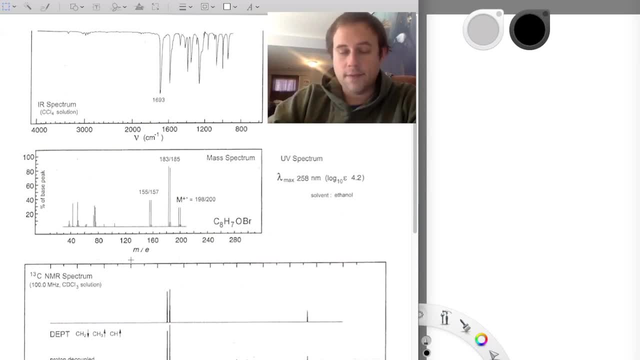 underlying theory. we're kind of assuming you have an understanding of that already. Okay, so let's take a look here. The first thing I do: I save my NMRs for last. They will give us the most information, but I gleam what I can out of the initial part up here. first And the easiest: 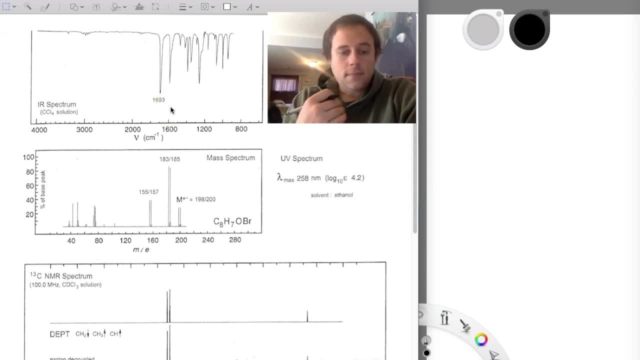 to start with is the IR. The IR does not tell you the specific compound that you have, not anywhere in the world. What the IR does is that it will allow you to identify certain functional groups. So remember, infrared spectroscopy will use infrared energy and it's going to stretch and 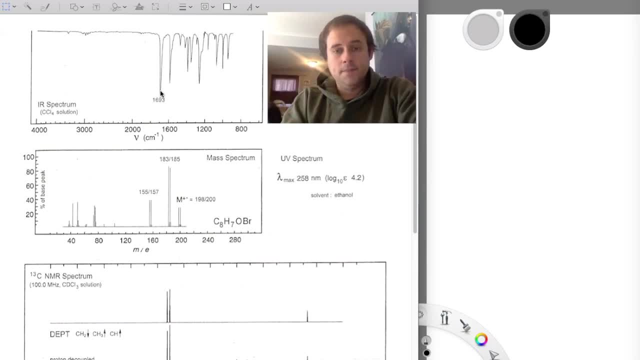 vibrate bonds back and forth at certain frequencies And so we can see the frequency down here in inverted centimeters as the scale, And that's typical for an IR when you're looking at it. And then we come along the top here and we see this peak right here Now. 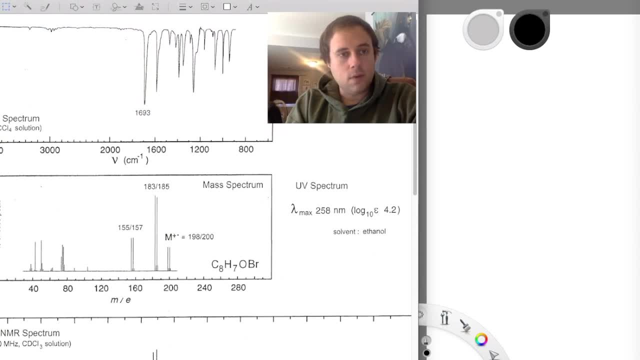 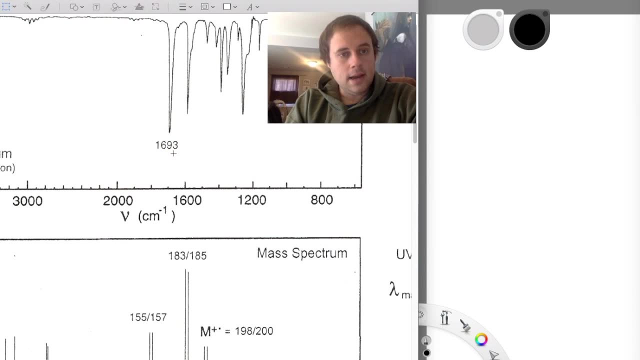 I'm just going to magnify this so that we can see as we're working with it, especially since we're sort of watching this on YouTube. We want to make sure everybody sees this- 1693.. So this peak- and note that usually as you start to go below 1500, not all the peaks are- I don't want to. 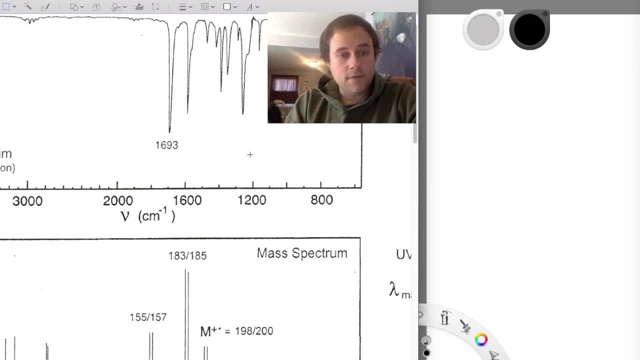 what term should I use? Useless, But that's known as the fingerprint region, and it tends to be crowded with a lot of unique peaks for each individual structure. IR is for And so while you can find some useful information down here, we tend to stick at. 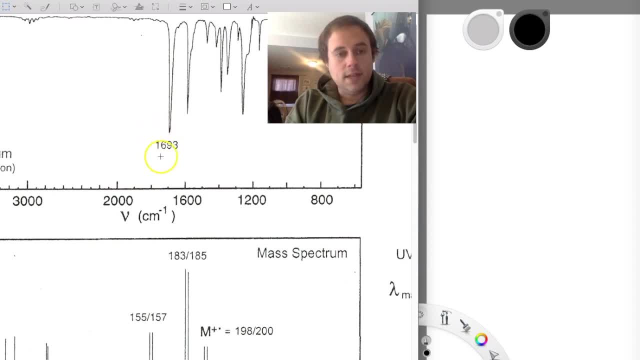 stretches that are above 1500 for most of the information, So 1693, and a sharp peak like this. this is most definitely indicative of a carbonyl. So what I'm going to do over on the right here if I can get my pad to focus, Okay. So for my IR, I'm going to note down that I have a stretch of 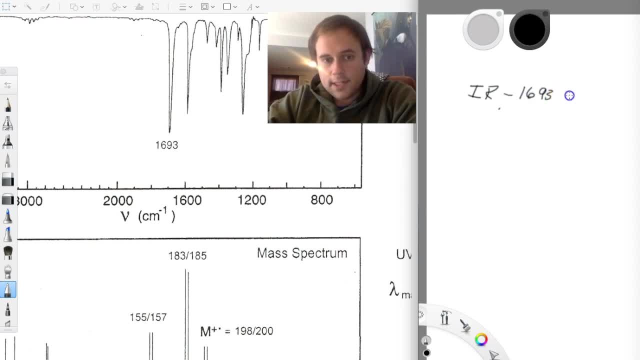 at 1693 inverted centimeters, And I'll just make a note to myself that that is most likely some sort of a carbonyl group. Now, yes, you could get more specific. You could start trying to say: is this a ketone and aldehyde and ester? I tend to tell my students not to focus on the IR, for 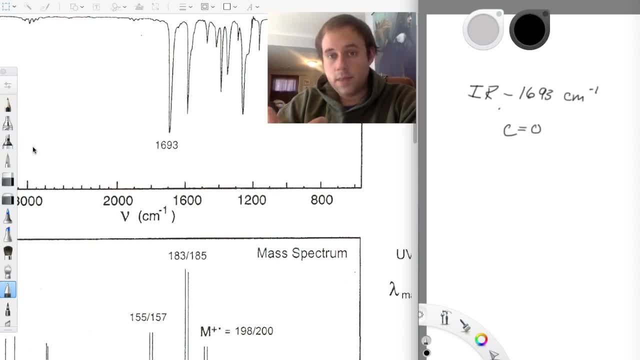 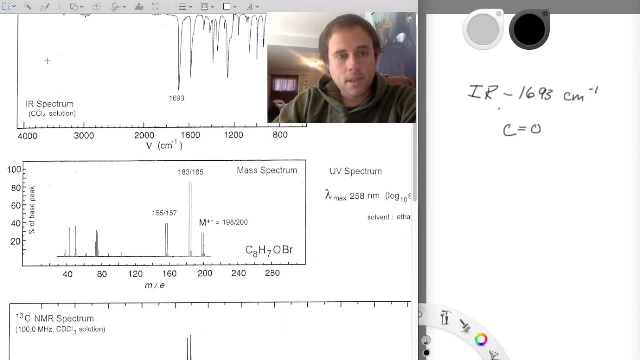 that so much because it should become clear as you work with the NMR. Now, sometimes the IR is good for that, So I don't want to completely play that down. All right, so that's primarily the critical information that we can get gather from this IR. 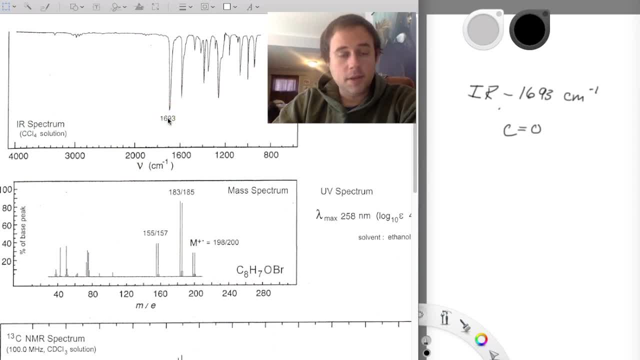 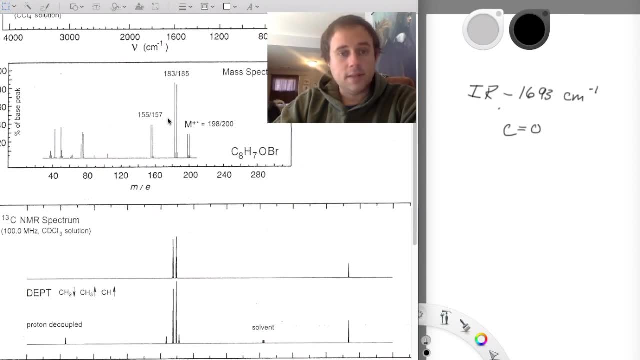 We only have one serious peak that's being labeled. for us that looks to be important. So, coming down to the math spec Now, there's a lot of various stuff you can do with math spec. A lot of students will focus on some of these other peaks that are further down here around the, you know, 40,, 80. 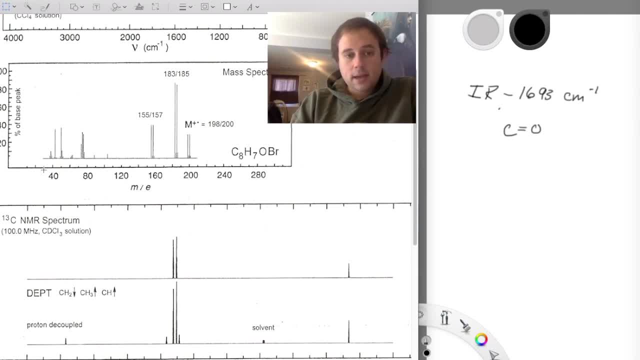 region, et cetera. The math spec is an instrument that when you place the, you inject the compound into it, it uses very high level electron energy and it basically fragments your compound into various fragments and then they go and they hit the detector. so 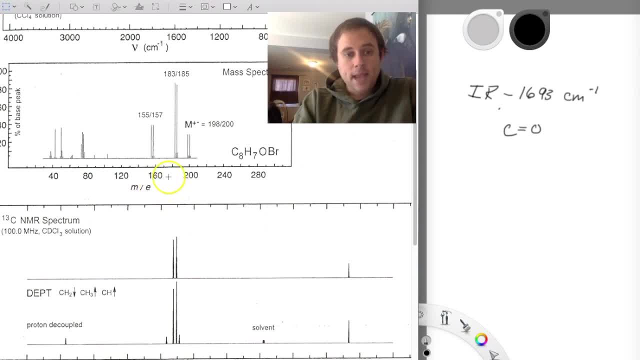 this is a mass to charge ratio M to E, and when you are dealing with this, these lines, all these different lines that you see, are different fragments that have basically been chopped off or cleaved off from your molecule that are hitting the detector. all right, for the sake of making this as simple as possible, 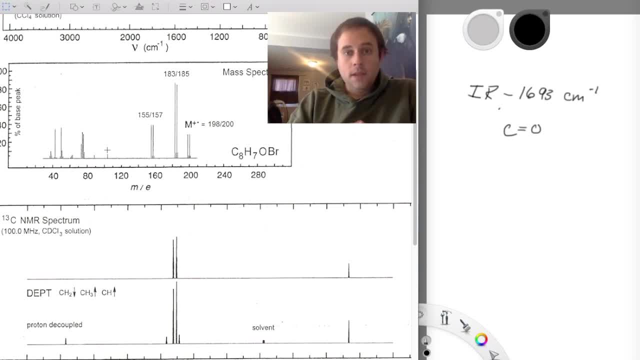 because you already have a lot of work to do when you're solving an unknown. these are the two major things that I would be looking for. so the first major thing here is that I would look for my M plus peak and the M plus peak is going. 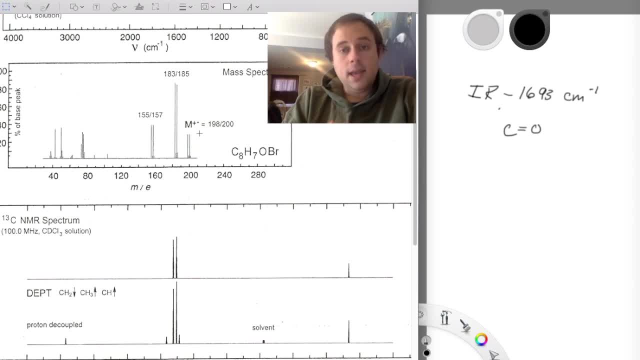 to be known as, essentially, the molecular ion peak. it is going to give you the molar mass of your compound. so we know that whatever we're working with based on the mass spec, let me move- so I'm just gonna move this- my pads a little better here, all right, so for the 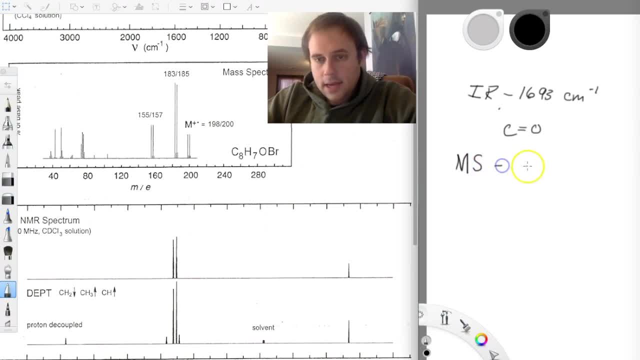 mass spec. I can take notes that my molecular formula is C8H7OBr, and then I'm also going to take note of the fact that it's 198. now notice it says 200 here: 198, 200 slash 200 grams per mole. so a lot of students will ask: what is that? well, 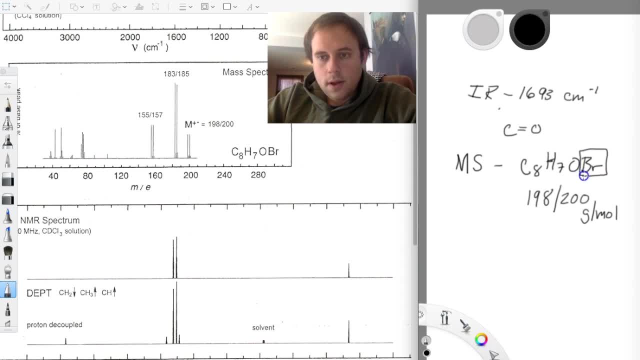 bromine has two differing isotopes and it just so happens that they're off by two grams from one another in terms of the molecular weight, and so, because it's in a one-to-one ratio, when you look at bromine here you have half of your. 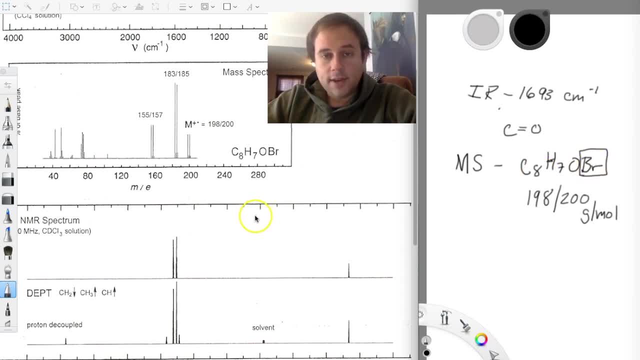 bromines, as the lower isotope bromine 79, and then the other half as the higher isotope bromine 81. so about 50 percent of all bromines in the sample will be 79, the other half will be 81, and so that's what leads to basically a 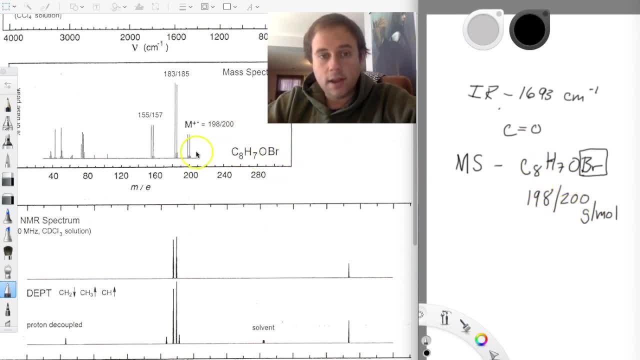 mixture between these because we have a bromine. this is very, very classic for a bromine to give these double sets of peaks like this when it's still attached to the molecule. so we very clearly have a bromine. that even says it in our our mass spec formula here. so one of the other things that's very 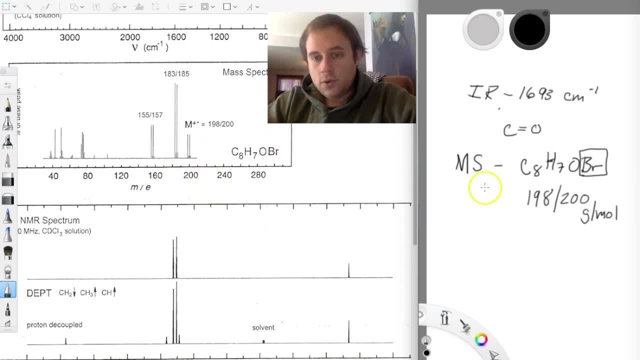 important to do, that you want to be working with is that you do want to attempt to calculate the degrees of unsaturation. so, for those of you that don't remember, this is usually represented by Omega, and degrees of unsaturation is the- the number of hydrogen's that are missing as compared. 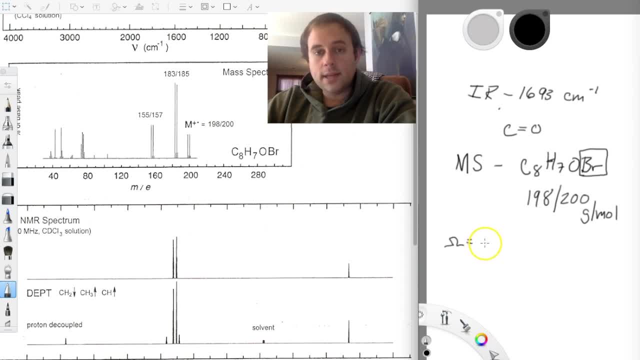 to when the compound would be saturated and full of hydrogen. so it can tell us a little bit of information about double bonds, rings, triple bonds, etc. so it's a good thing to keep tabs on because it will place limits on us when we attempt to solve for this structure. so 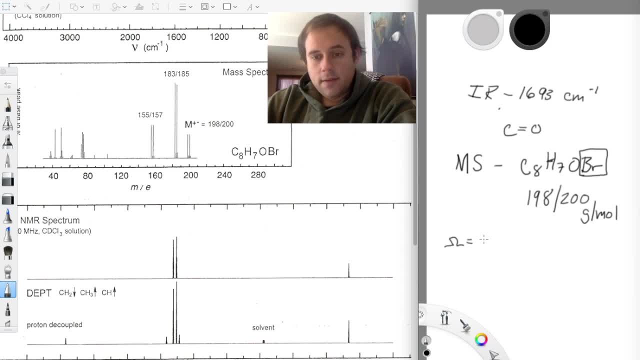 if we take a look at this, the formula for degrees of unsaturation is 2n plus 2 minus X over 2. now n is the number of carbons, so it's going to be 2, and the number of carbons here would be 8, and then plus 2 minus now X is going to be. 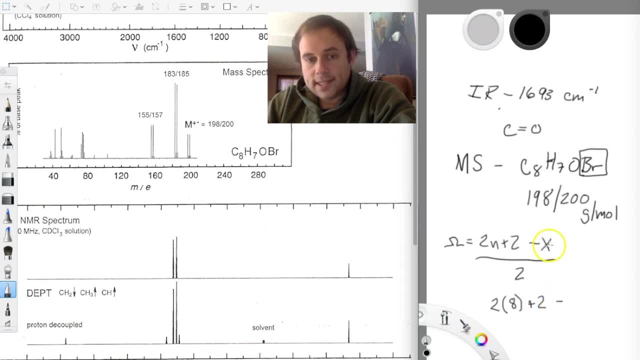 equal to the number of hydrogen presence. so in this case it's 7. you have to consider the fact you have an oxygen and a bromine. oxygens are completely ignored when calculating degrees of unsaturation. however, bromines are going to add one to your total running number of hydrogens. they act. think about how a 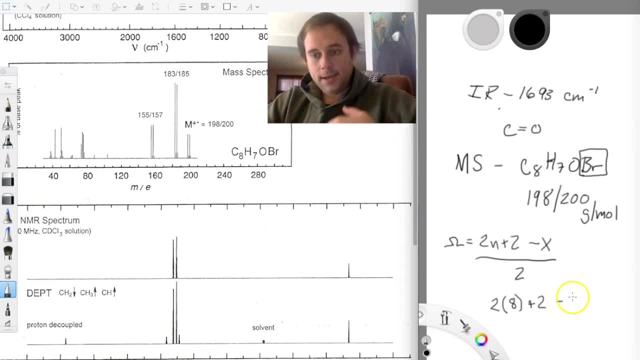 halogen bonds to carbon. it basically forms a single Sigma bond with most carbons, and so it's behaving in a similar fashion as hydrogen bonds with carbon hydrogen would, So we will count for it as if it's behaving as a hydrogen. So instead of minus seven, 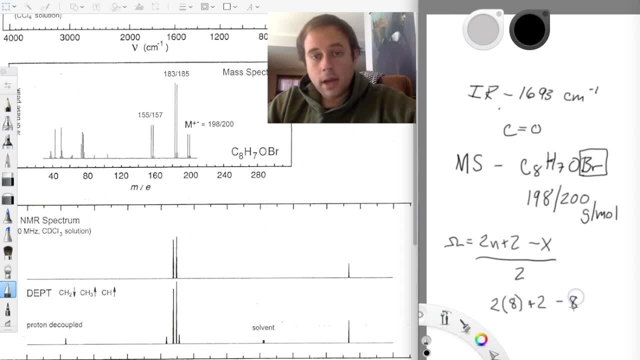 it's going to be minus eight And, by the way, if we had a nitrogen present, it would take one away from that hydrogen total. So this is what we're working with, and then we would end up dividing this by two, Okay, and that is going to give us the degrees of unsaturation. So, if I take a look, 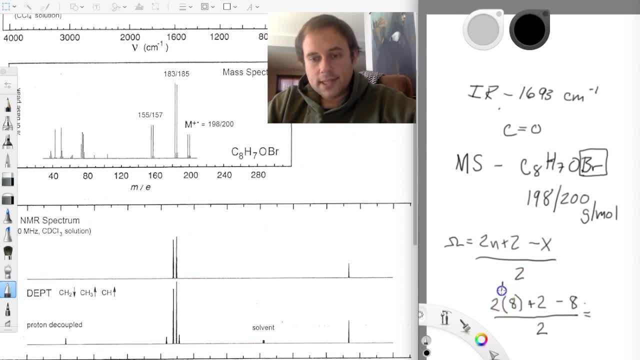 at this here: two times eight is going to give me sixteen plus two is eighteen. So eighteen minus eight is going to be ten. divided by two is going to be five degrees of unsaturation. That is a lot of unsaturation. So one degree of unsaturation can be equal to a double bond or a ring. 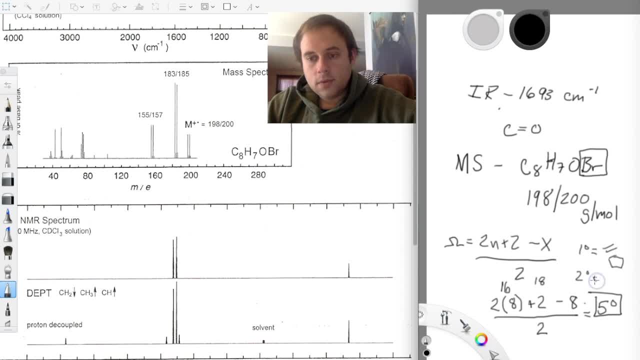 And and and. the two degrees of unsaturation can be equal to a triple bond or any combo of two of the single degrees of unsaturation. So I could have two double bonds, two rings fused together: a ring and a double bond, one triple bond, so on and so forth. Now, one of the tips that I have, and this isn't always the- 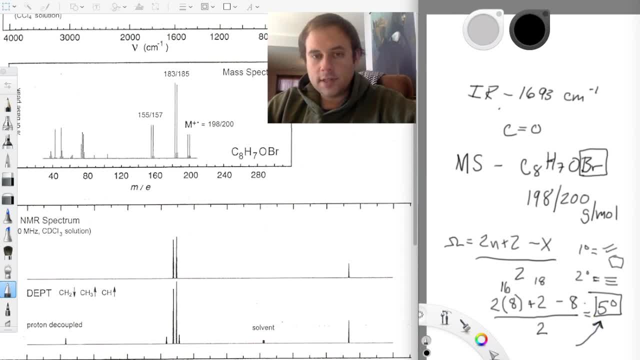 case, but it usually is- If you have four degrees of unsaturation or higher. many times you're dealing with a benzene ring, because that is a lot of degrees of unsaturation. So a benzene ring requires one degree of unsaturation for the ring and then another three, So a total of four degrees of. 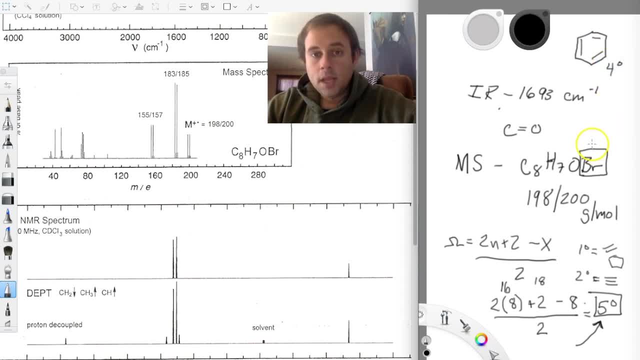 unsaturation for the entire ring itself. So when you get up to five degrees of unsaturation, you're probably not dealing with a compound that has, you know, two triple bonds and one double bond, or five double bonds, or a system that has five rings fused together. You might, but those would be pretty. 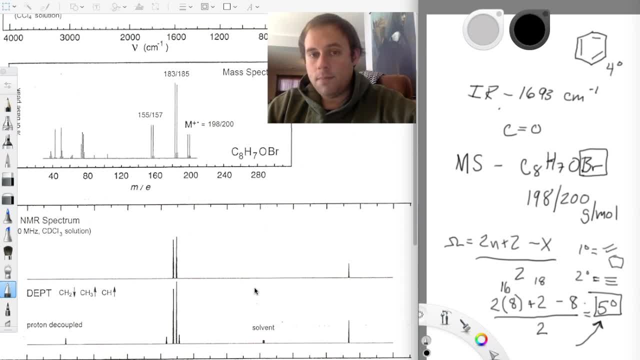 complicated Examples for an undergraduate class. So I would most likely think that you would have an aromatic ring and we're going to be able to confirm that when we go down and we start looking at the carbon NMRs and the pro, especially the proton NMRs, will show if we have some aromatic ring activity. So this is useful. 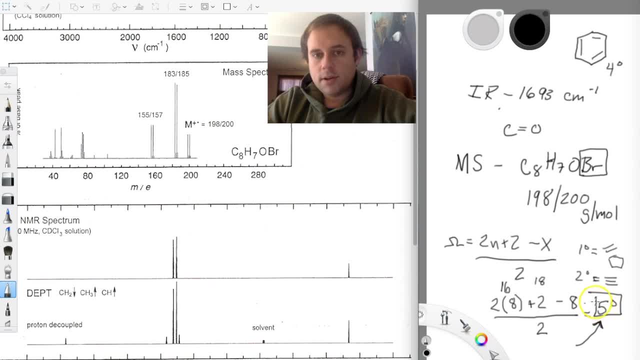 information OK, Because it places limits on the number of double bonds, rings, triple bonds, etc. that we can have. So this would be the first half of how I would attempt to solve this problem. Now I will also need to work with some other people to try to solve an unknown problem. I would get my IR data. 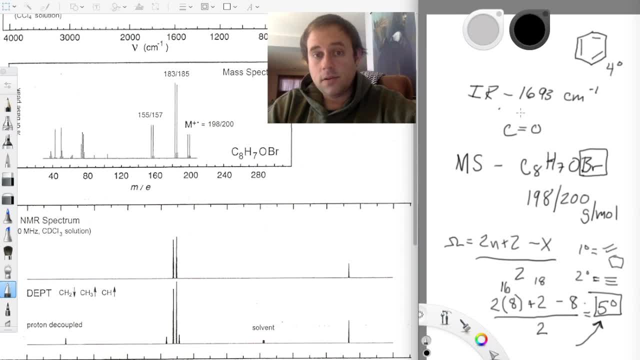 and then I would also collect any data that's relevant from the mass spec, particularly the degrees of unsaturation. And this formula here, C8H7OBr, is going to be very important because that will tell us how many carbons, hydrogens etc. we have to work with. So when we're proposing compounds, they have to fall. 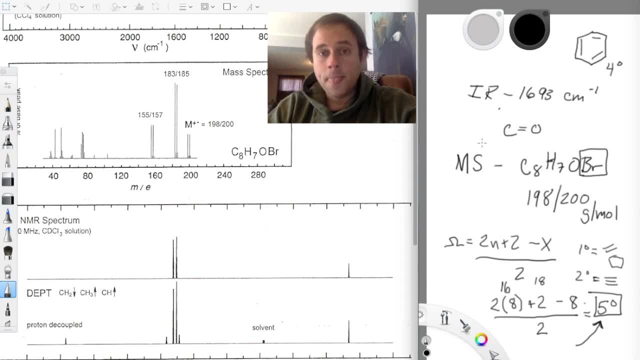 within this realm. Right, They have to take up five degrees of unsaturation, and they also are going to have to contain only eight, eight carbons, seven hydrogens, an oxygen and a bromine. Okay, so up next is the carbon NMR. 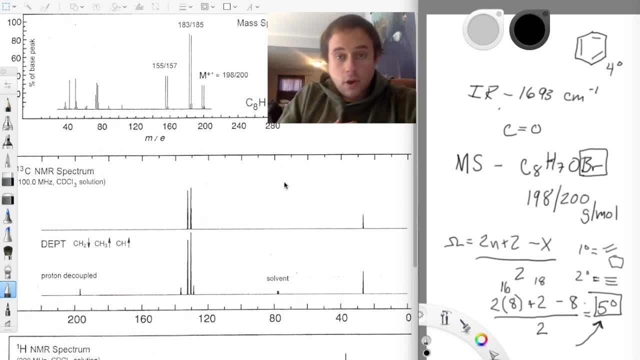 Carbon NMR is useful. However, my personal opinion is carbon NMR is not as useful as proton NMR. Proton NMR tends to give us more detail about the skeletal structure of the compound. However, carbon NMR can be very useful. 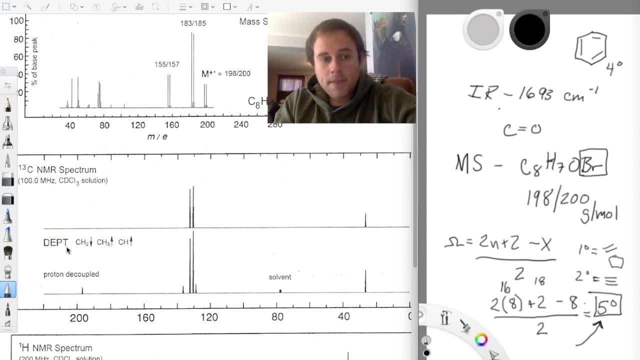 So right here we have something called a dept carbon NMR. Dept carbon NMRs will show carbons that have protons or hydrogens associated with them. So this is not actually showing the protons. It is showing the carbons that contain protons. 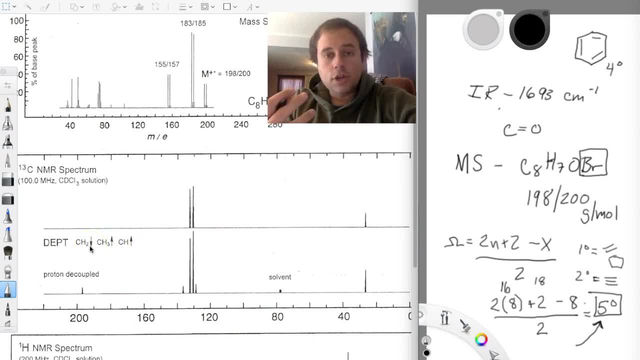 Okay, and one of the cool things about the dept NMR is that it will show any methylene groups, CH2 groups, inverted on the axis of the dept, And the CH3 and the CH groups are going to appear on the upward portion. 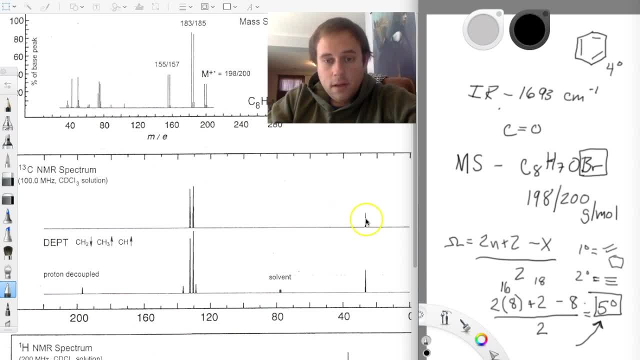 So what we can see? What we can see here, is that I have all these peaks facing up, So that means there are no CH2s found anywhere in my molecule. So if you have a dept NMR, it can be very useful in sort of eliminating or confirming whether you have CH2 groups. 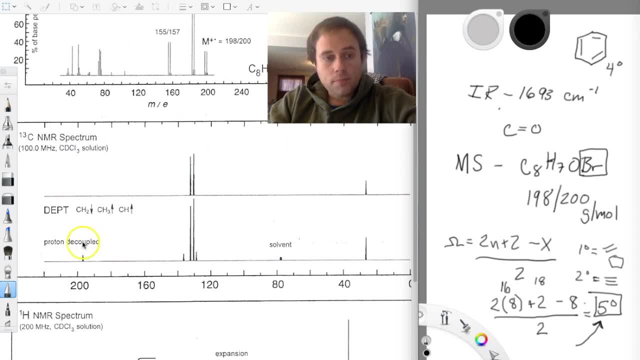 methylene groups present. Okay, and then we go to a proton decoupled, meaning that we are not allowing protons to create any sort of coupling or splitting. That's going to occur here And we can take a look at the number of peaks. 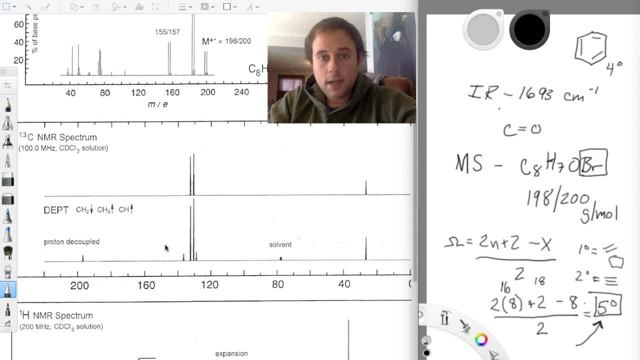 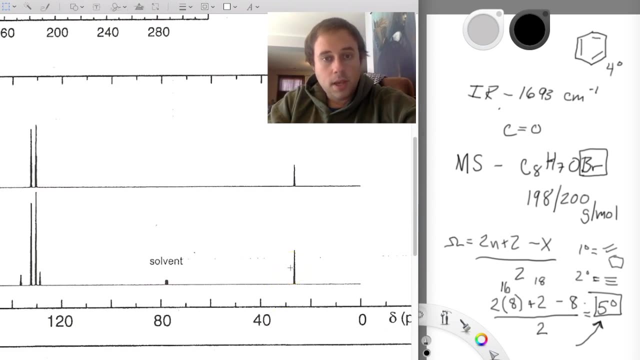 And that will be associated with the unique number of carbons in our molecule. So take a look here. I've got one over here And if you look carefully, maybe we'll zoom in on this again. All right, So I've got right here upfield. I've got this one peak. 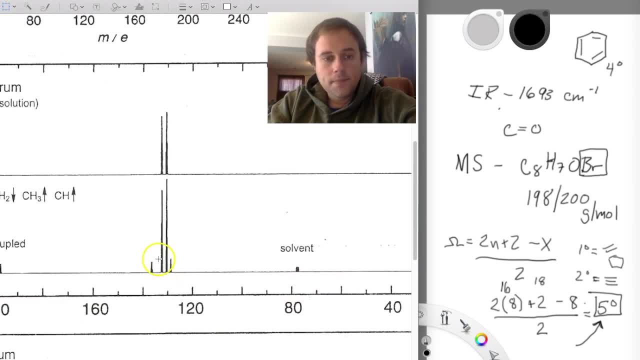 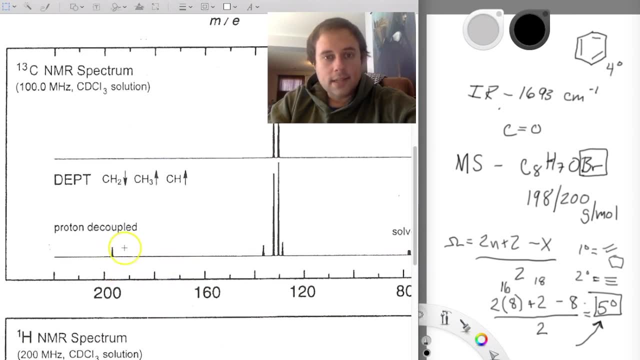 I ignore solvent, I'm not worried about my solvent, And then I've got four of them here, So that's a total of five. And then all the way up here I see six, So that's pretty high up. Okay, so I have six unique carbons that I need to account for total when I'm dealing with this structure. 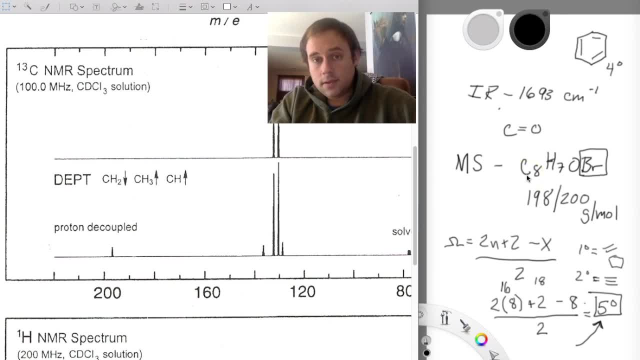 Now, keep in mind I have a total of eight carbons in the structure, So that means some of the carbons are not going to be unique. They're going to be identical or symmetrical to one another. magnetically identical, Okay, because, remember, NMR uses magnets. 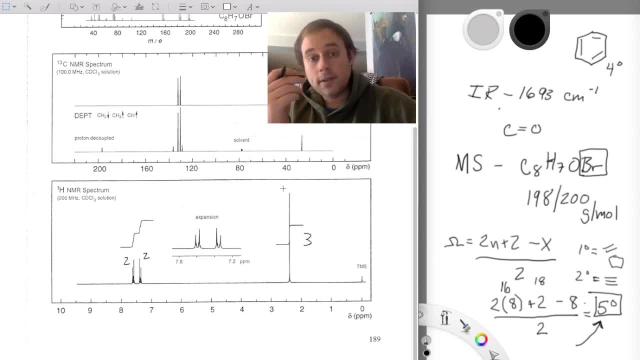 Takes advantage of the fact that nuclei are essentially little magnets that are spinning on their own axis And we get them to align and interact with a larger magnetic field that's being generated by the NMR instrument. All right, So what I'm really focused on here- and there is a little more you could sort of gather out of this in terms of the chemical shifts. 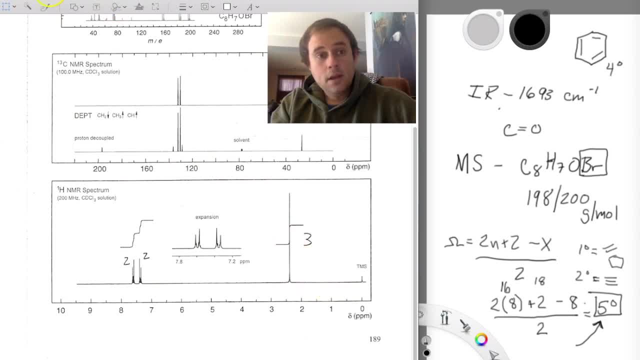 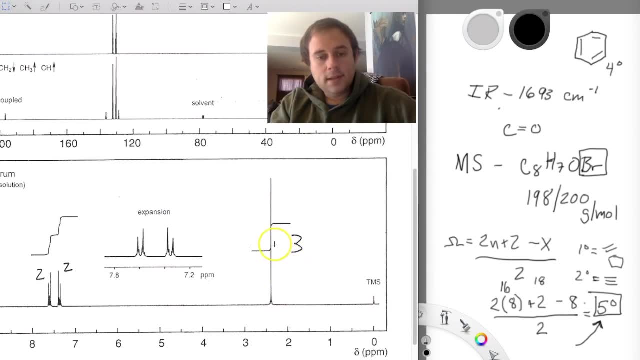 But I really would rather focus on the proton NMR to do that. So here's what I've got. All right, If I take a look at my proton NMR, I have this peak which is appearing as a singlet around 2.4 approximately. 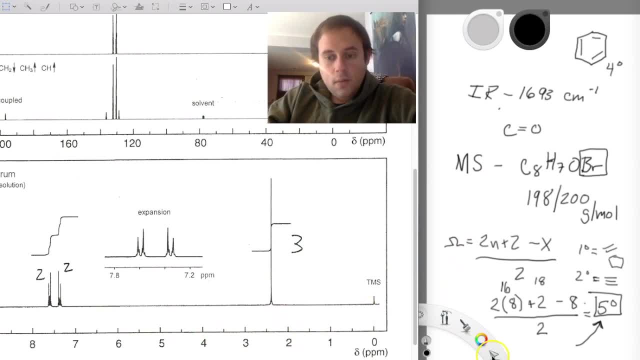 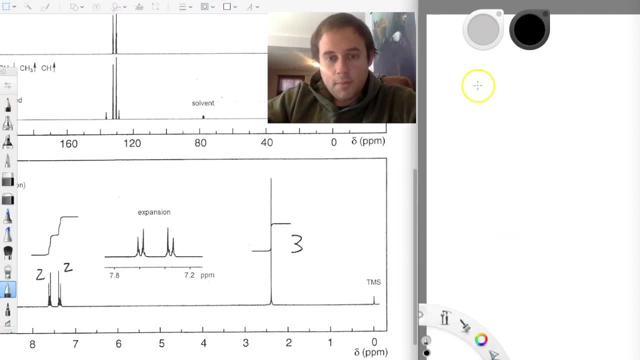 And it's integrating to three. All right, So when you start, make sure you have this copied down. I'm about to delete, Okay So, because I want to make some NMR notes here. So the first thing that I'm going to mention is that the C13 told me that I have six unique carbons. 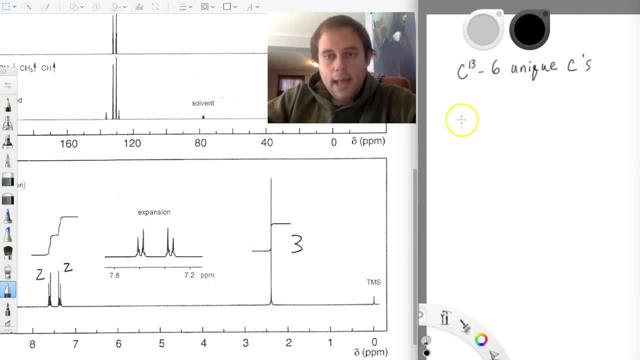 And then the H1, I'm going to start analyzing it here. Oh, we can also mention up here, right, that we have no CH2 groups. That's important. So the H1 that I have here, The first thing I see is I see a singlet. 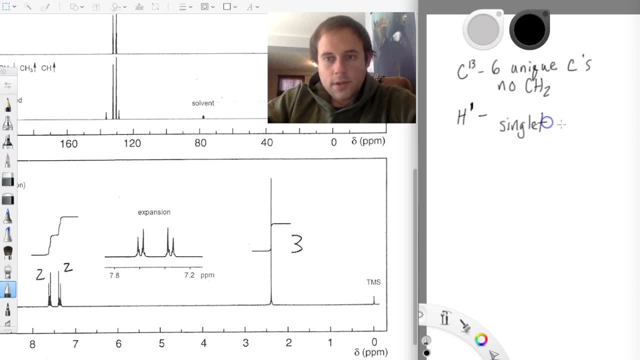 That is going to integrate to three Right And it's got a ppm of around 2.4 ppm. So what can I gather from this? Well, I know that whatever this signal is associated with, it's associating with three protons. 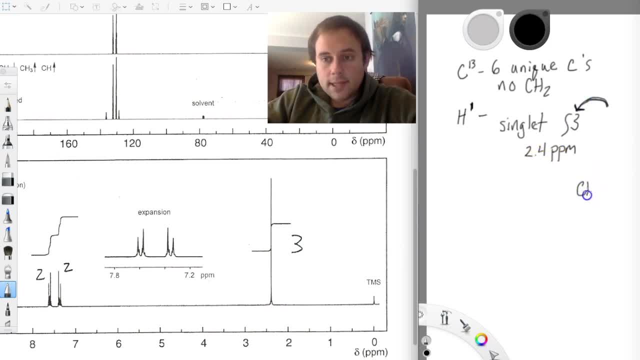 And so, most likely, I would say that this is a CH3.. Right, That's going to make the most sense. It's a singlet, So whatever the CH3 is next to, it has no neighboring hydrogens, Right? So we don't know what this is attached to. 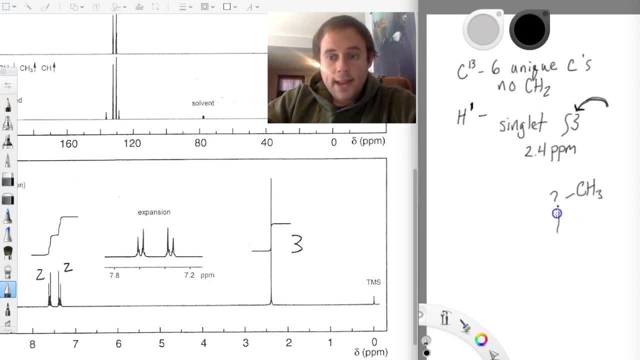 Most likely it's a carbon, But what we do know is that the neighbor here is going to have no hydrogens Because it's not splitting Right. So remember, the general rule for splitting is N plus one of the neighboring protons. 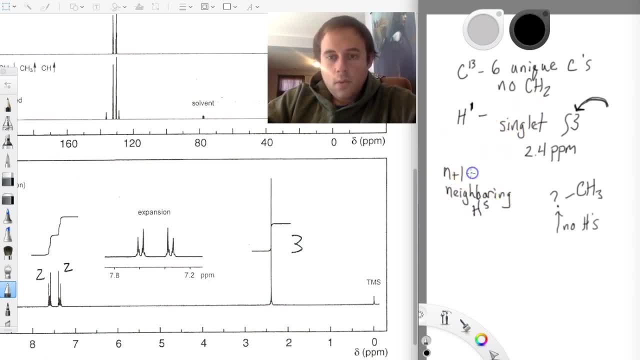 So if I look at N plus one in order to get a singlet which is one peak, then N would equal zero Right, Right, Right, Right Right. So that means the neighbor, which again we're going to assume is a carbon, is not. 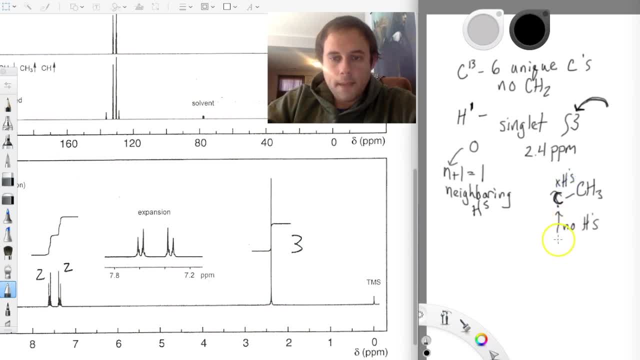 going to have any hydrogens associated with it. Right, So I can come back to this in a minute. The chemical shift is going to be important. If I take a look at it, regular methyl groups are going to appear somewhere probably between like 0.7 to maybe 1.2 at the highest. 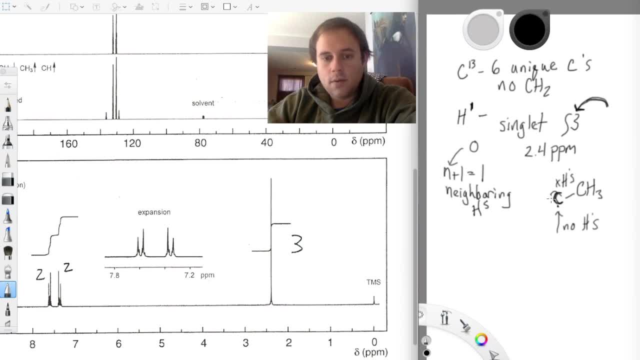 And this is quite a bit above that. So I've got a PP. I've got a PPM of around 2.4 when I'm looking at this, And if my PPM is that high, it's most likely due to some electron withdrawing group or 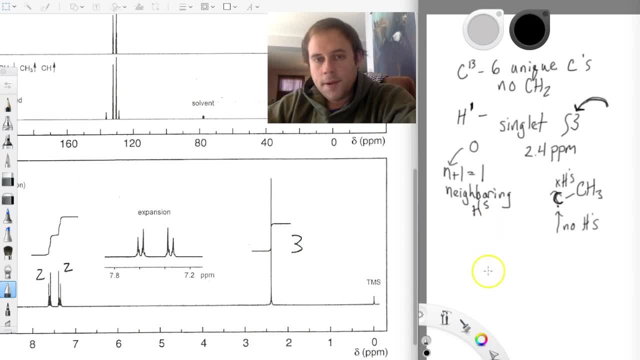 electronegative group that is in the proximity of this methyl group. So at this point I would think, OK, well, what could be there? Well, I do have an oxygen And I already know what the oxygen is associated with. 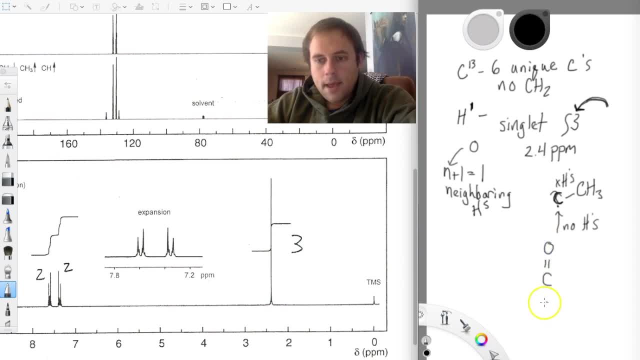 It's associated with a carbonyl And I also have a bromine. Those are really the two primary Electron withdrawing groups I have. I did mention that I may have an aromatic ring And in fact I can confirm here that I do have an aromatic ring, because in the region of 7 to 8 PPM. 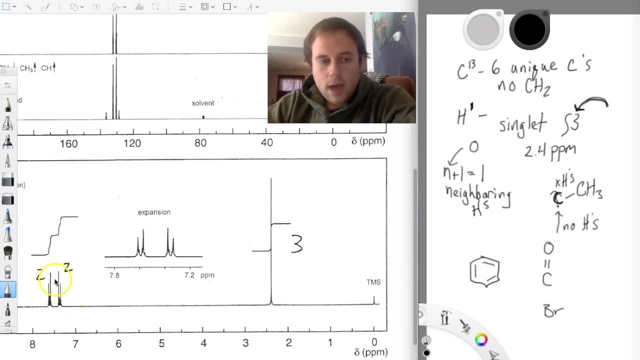 that is where aromatic rings pop up, And so I can definitely confirm now that I do have an aromatic ring. The IR showed that I do have a carbonyl, And so if I take a look at this, this is four degrees of unsaturation. 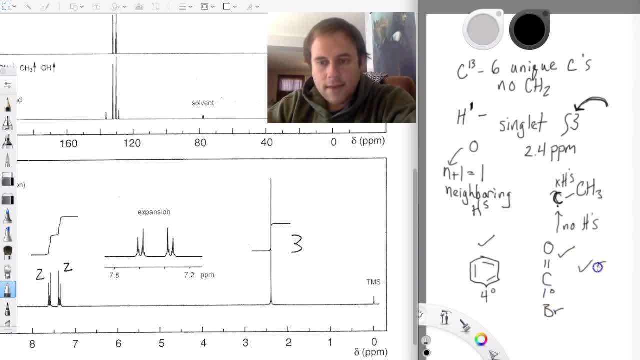 This is one degree of unsaturation. I have now Counted for all five degrees of unsaturation. So I have a bromine, I have a carbonyl of some sort and I have an aromatic ring. So that's not too bad. 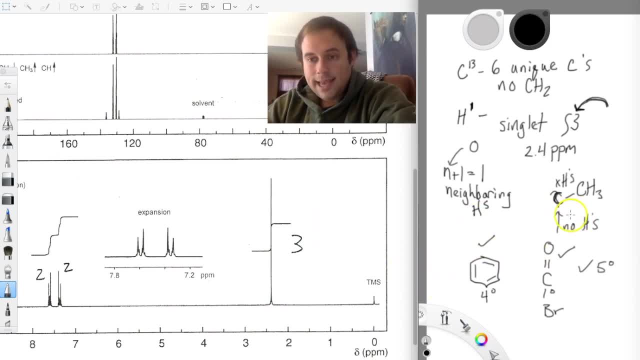 OK, All right, Continuing to put this puzzle together as we're working with this. So let's come back here. If I take a look, This CH3.. What could it be next to? Well, I could have a CH3, potentially. that's coming directly off of the aromatic ring. 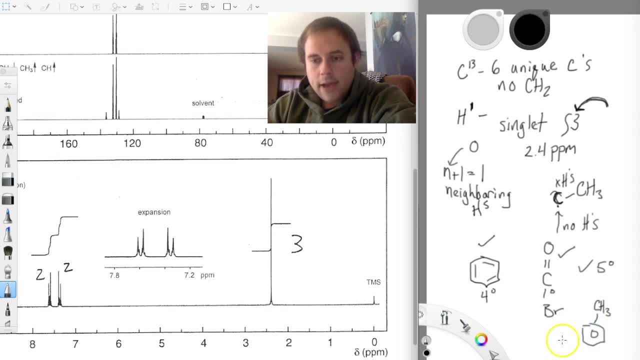 Right, I could have a CH3 that's next to a carbonyl group like this, Or I could consider the CH3 with the bromine. Now, the first one that should be out immediately is the CH3 next to the bromine, for two reasons. 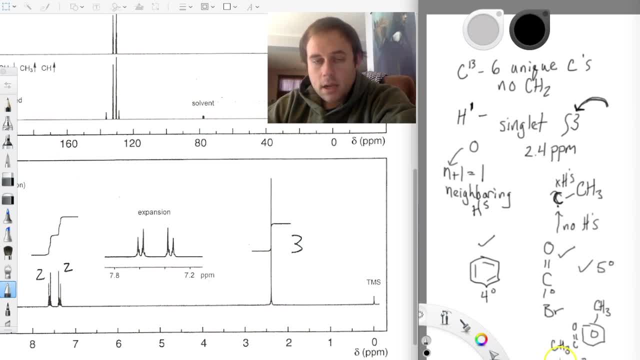 Number one. if I put CH3 and bromine together, that is a valid Lewis structure within itself. There's no room for the aromatic Or for the carbonyl in here, So this would eliminate the possibility of me bringing in the other needed structures for my unknown. 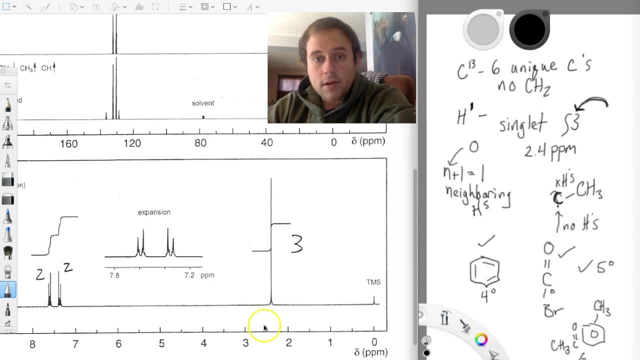 So that's out. The other reason that's out is that halogens have a very strong withdrawing effect And they would most likely show something around 3 ppm or further. downfield 2.4 is a little bit too weak for halogen electron withdrawing. 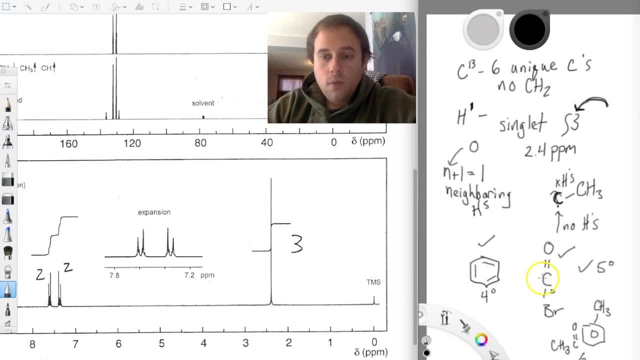 So that leaves me with the carbonyl and the aromatic. So what I'm going to go ahead and do at this point, I'm going to look at what I potentially have on my aromatic. So, looking at the aromatic system, here I have two signals. 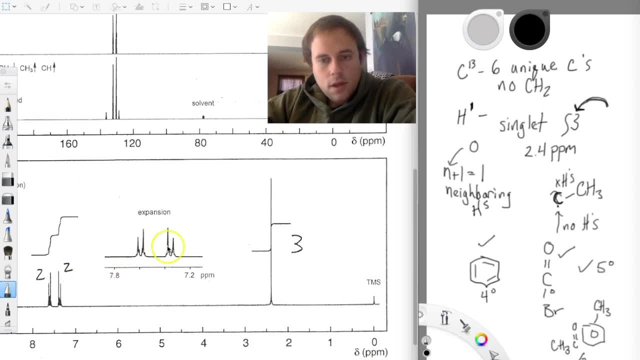 They both split into doublets And they both integrate to two. So what that means is that I have two sets of hydrogens that are identical And I have to have another two sets of hydrogens that are identical. So right now, all four of these are identical. 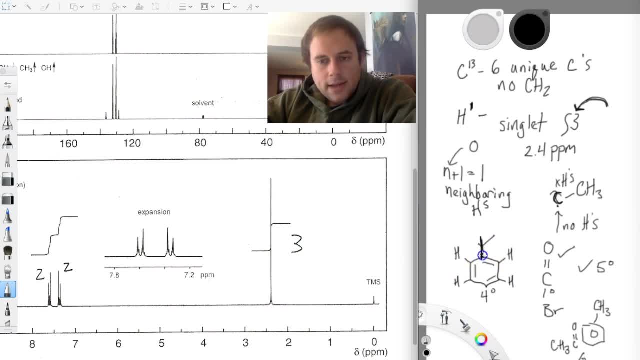 The key here Is that I'm going to have one group That's not hydrogen- We'll label that as X- And another group Coming off of here That's not X And also not a hydrogen, So we can label that as Y. 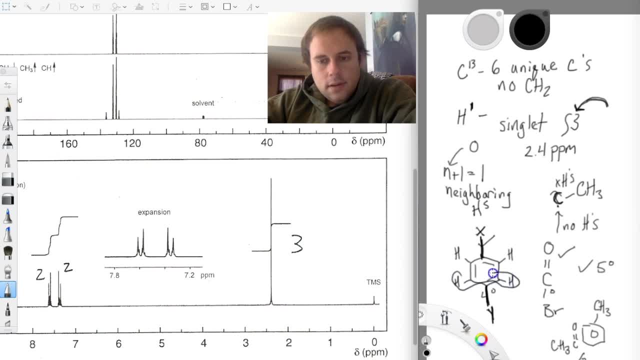 Then these two hydrogens Are going to be one space away from Y And two spaces away from X, Whereas these hydrogens Are going to be one space away from X But two spaces away from Y, So they're magnetically equivalent. 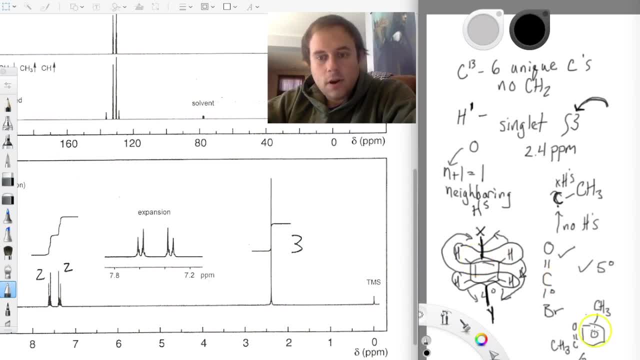 And they're giving rise to one signal. That's where our symmetry is coming from, With the carbons and the protons here. So let's clean this up a second. And what I've just determined Is that I've got an aromatic ring. 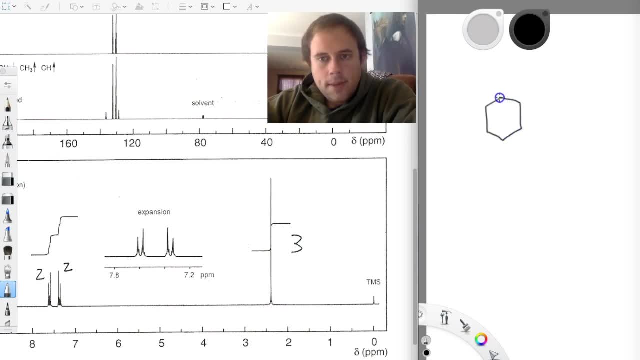 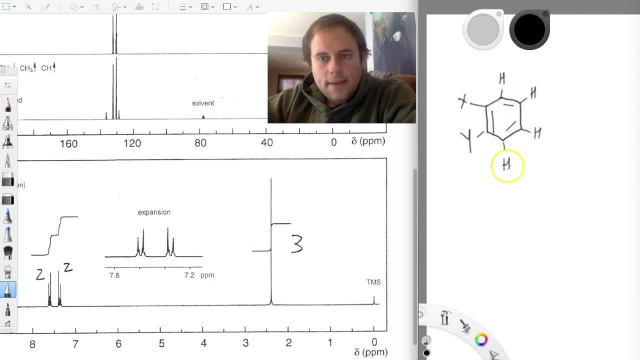 And Y. I don't have the same Identical setup here, Even though these guys Are both one position away. One of them is one position away from X, The other is one position away from Y, So they're not magnetically equivalent. 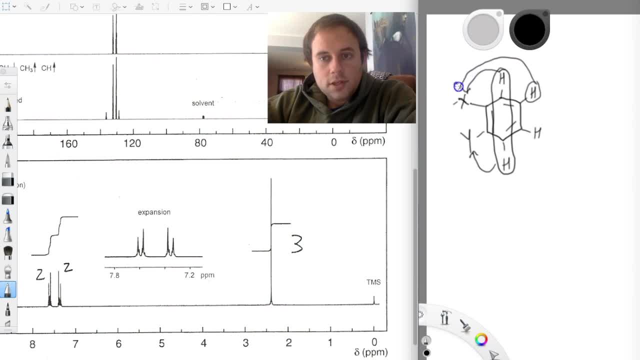 And this one Is going to be two positions from X And three positions from Y, Whereas this one would be Two positions from Y And three positions from X. So you're basically going to get more signals down here. You're going to destroy some of the symmetry. 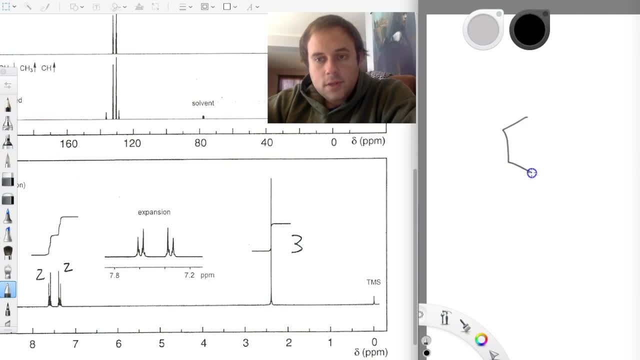 If you try to do that. So we know that the substitution pattern here Must be What we would call para, And so I have to have A one four Type of substitution pattern. I have an X and a Y, And that will make these guys. 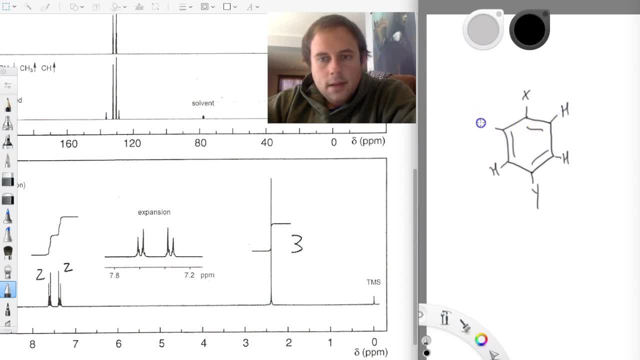 Magnetically equivalent And these guys Magnetically equivalent, Alright. so I want to try to start wrapping this up here. So then I say, okay, Well, what could possibly be on the ring? Well, we know the bromine is not going to be. 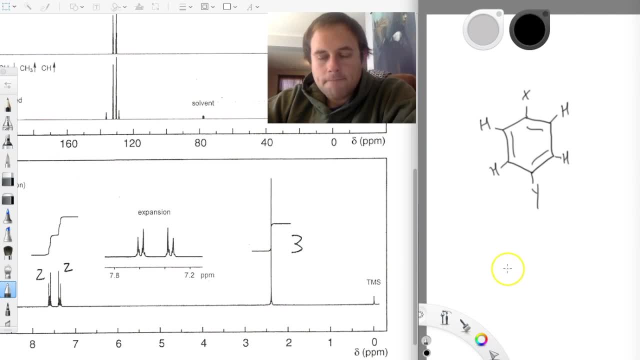 Attached to the. What do we say To the methyl group? right? So bromine Is most likely attached to the ring then, Because it doesn't have a whole lot else to go off of. That means That what I'm left with is a CH3.. 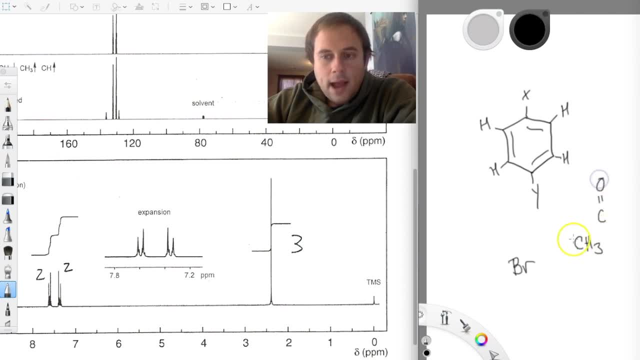 And a carbonyl. Now I cannot put three different substituents On this ring And outside of that I would need something On the other side of this carbonyl. Okay, The idea of acid bromide. So a BR that's coming off of the carbonyl. 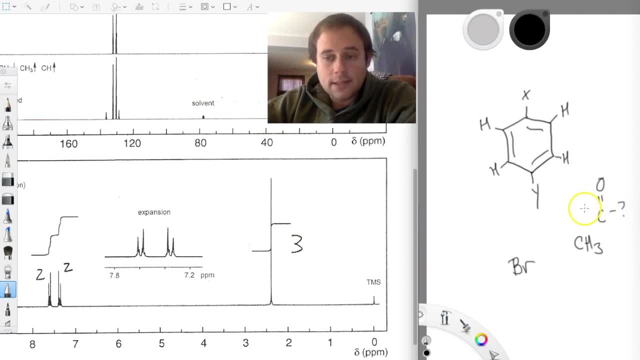 They tend not to occur very readily. Sometimes you can get acid chlorides, But acid bromides tend to be pretty rare. And on top of that, If we take a look at this CH3 here, It really is in the range Of. 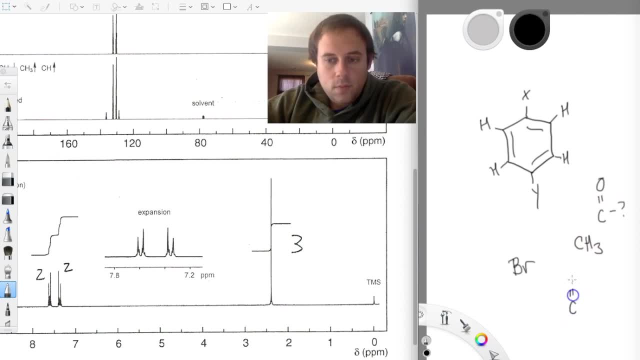 What would be associated with A carbonyl group. So we definitely have some sort of a methyl ketone here, Because These guys tend to show up in a PPM range of about 2. To 2.5. Depending on what's on the other side here. 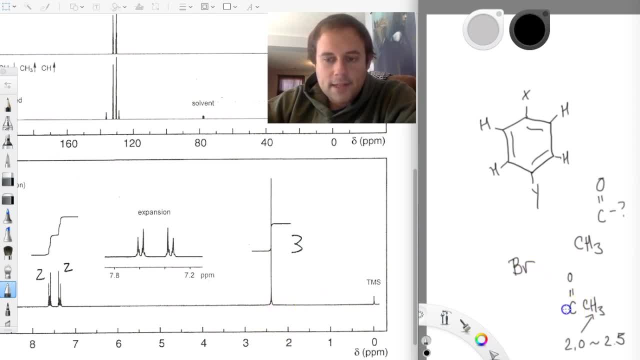 And so this falls perfectly within that range. So what I probably have is a Methyl ketone On one end of the ring And a bromine on the other. So that's what I'm going to propose. Okay, I will propose that I have a ring. 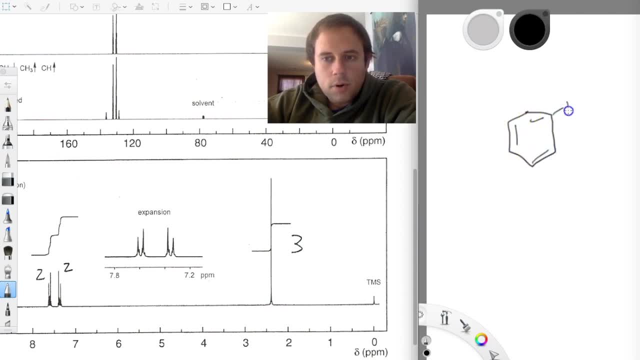 This ring Would have four protons In these positions, And then One side of the ring- Doesn't matter which side you pick out to draw this on- Is going to have The methyl ketone And the other would have the bromine. 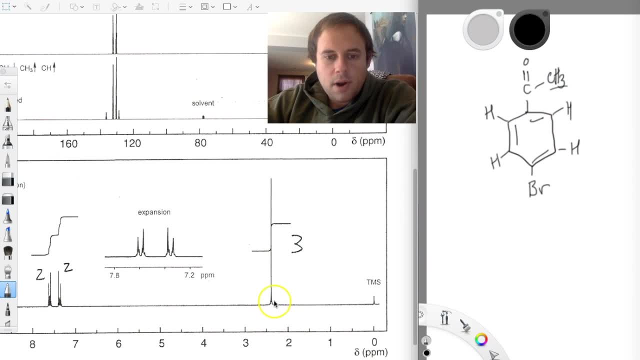 So does this make sense? So if I take these two And I divide them into three And it shows up in the proper PPM region, These would integrate to two. And they show up in the aromatic region And these integrate to two. 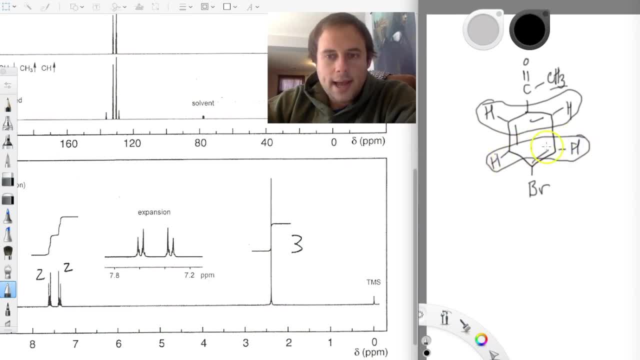 They also show up in the aromatic region And notice the splitting here. These are treated as one signal, And so the neighbor. There's one neighboring hydrogen. So one plus one, Because it's n plus one equals two, So these appear as doublets. 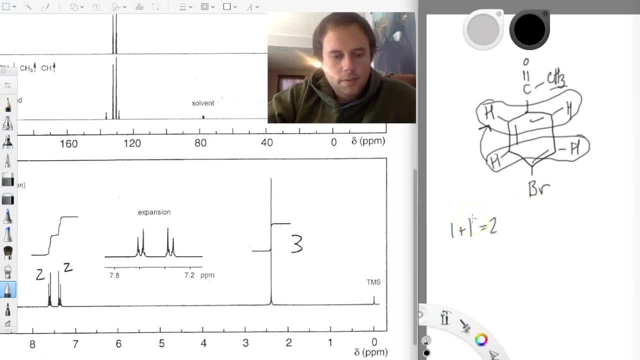 When I'm taking a look at them. So let me just Clean this back up So we can take a look at our structure. Alright, so this is the structure we're working with. Now For the final check. You should always go back and check yourself.